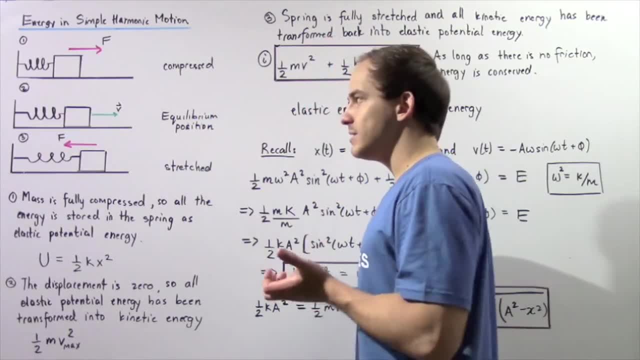 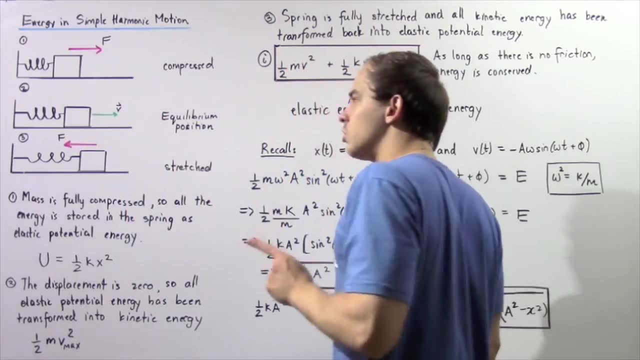 So because displacement is zero, that means that the force acting on the object due to our coil spring at the equilibrium position is also zero. Now that means our object will have a certain force acting on the object due to our coil spring at the equilibrium position. 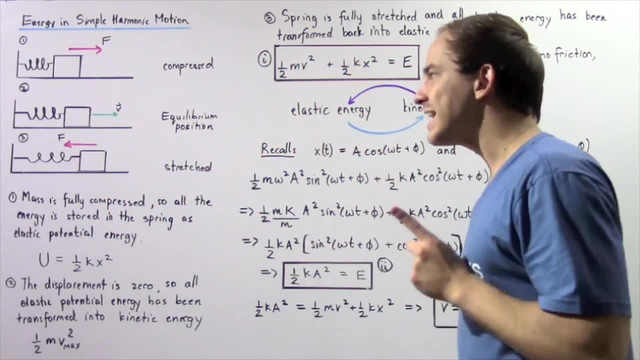 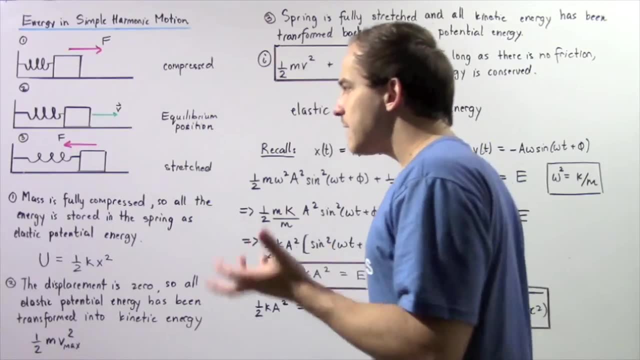 So, because displacement is zero, that means our object will have a certain velocity and that velocity will be the maximum velocity that our object can reach during its harmonic oscillation. Now, eventually, the object will reach a stretched position where the spring will be completely. 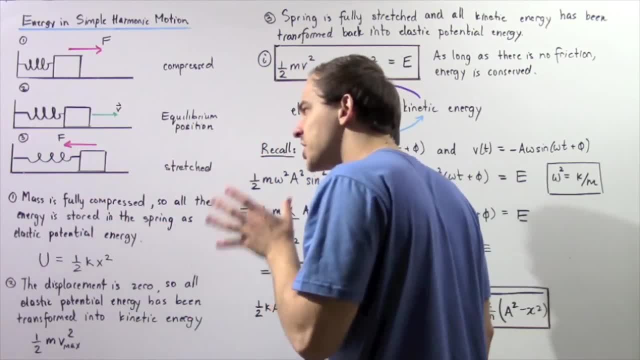 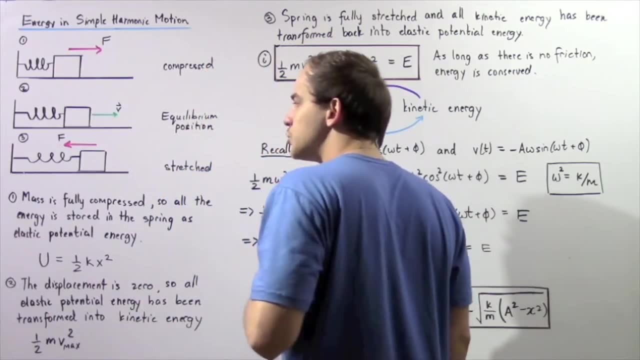 stretched And at that point the object will momentarily come to rest and the force will act in the opposite direction of our motion, So it will point in the negative direction of our motion And at that point the force acting on our mass due to our coil spring will accelerate our object in the 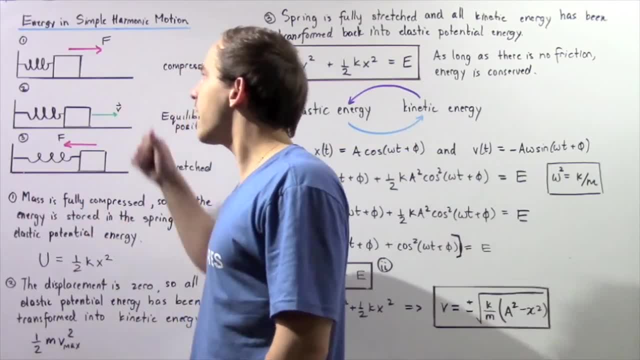 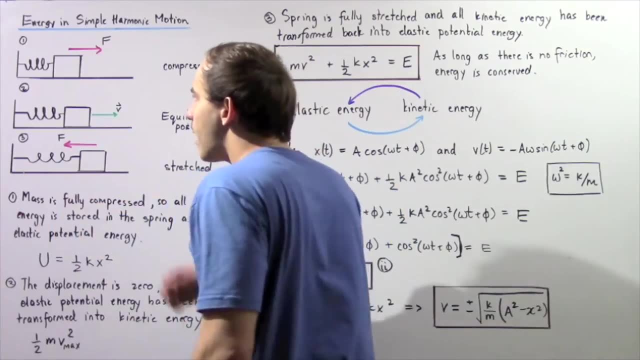 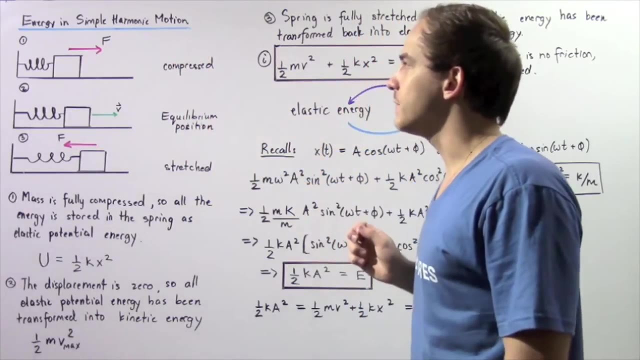 negative direction along the x-axis, bringing our object back, restoring that object back to its initial position. So the object will continue to oscillate back and forth. Now let's talk about the energies of these objects in diagram 1,, diagram 2, and diagram 3.. So initially in diagram 1,. 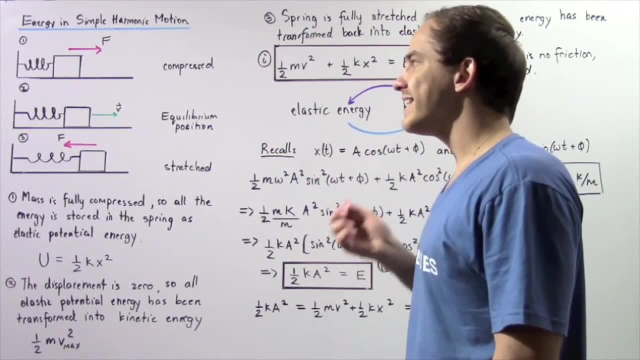 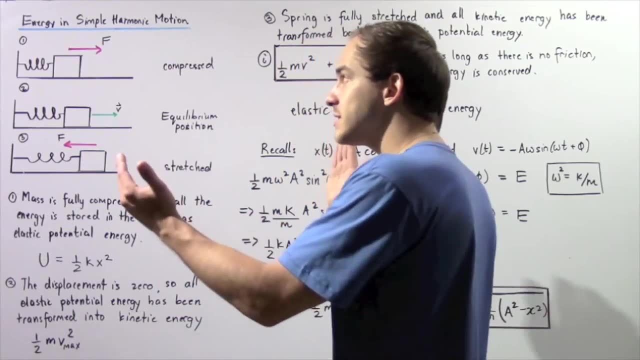 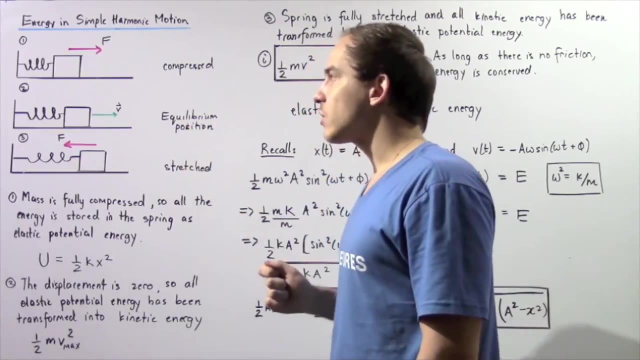 our object has no velocity, So that means it has no kinetic energy. But the spring, the spring is compressed, So that means, because the spring is compressed, a displacement. that implies that there is energy stored in our spring as elastic potential energy. So in diagram 1,. 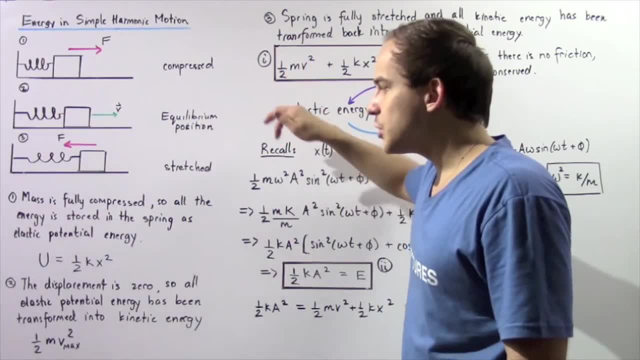 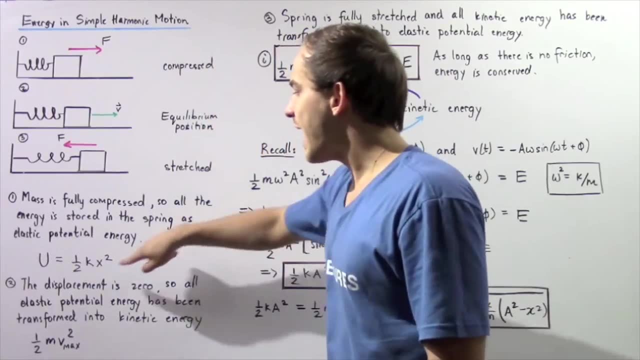 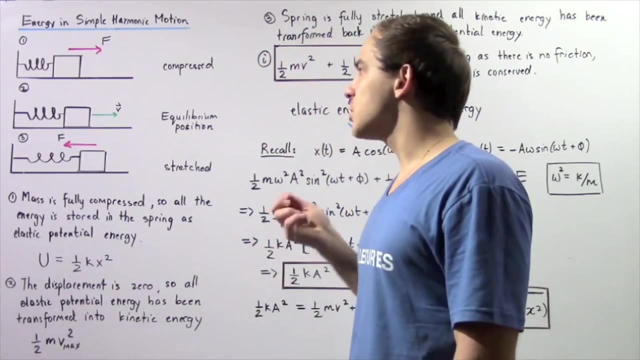 the mass is fully compressed. so all the energy is stored in the spring as elastic potential energy and it's given by this equation, where x, in this case, is our amplitude. So this equation gives us how much elastic potential energy is stored in our spring that is compressed — a distance. 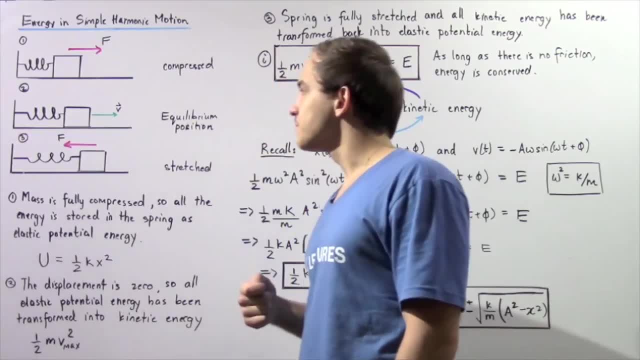 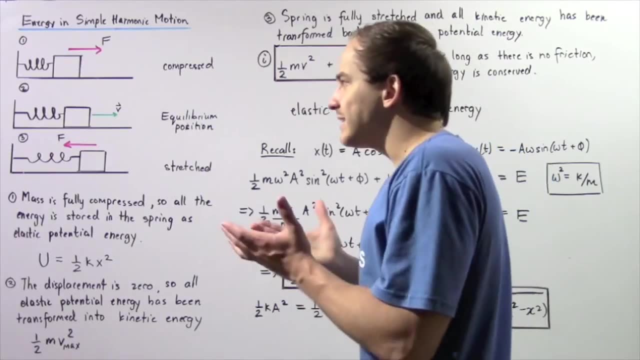 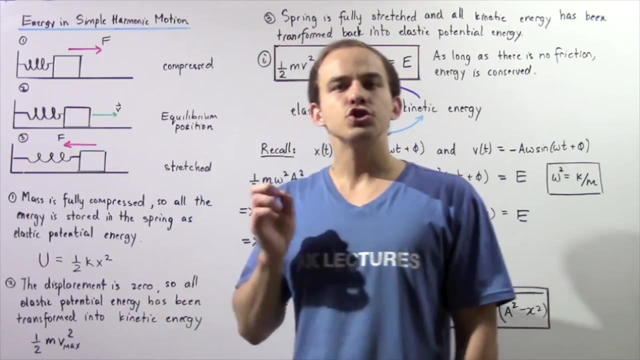 x and has a spring stiffness constant k. Now what about position number 2?? Well, in position number 2, our spring is not compressed and it's not stretched. The displacement of our spring is 0, so that means there's no elastic potential energy. So all the elastic potential. 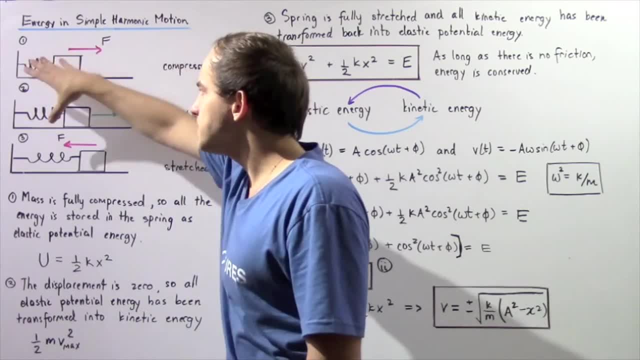 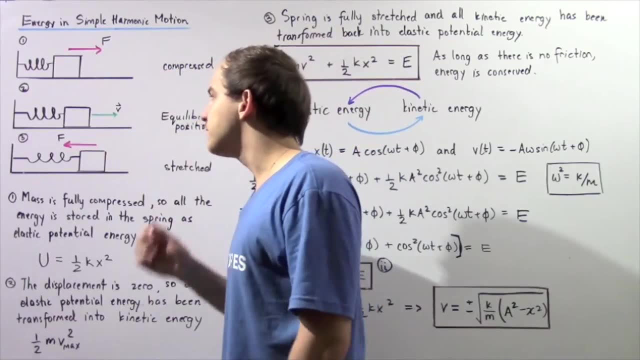 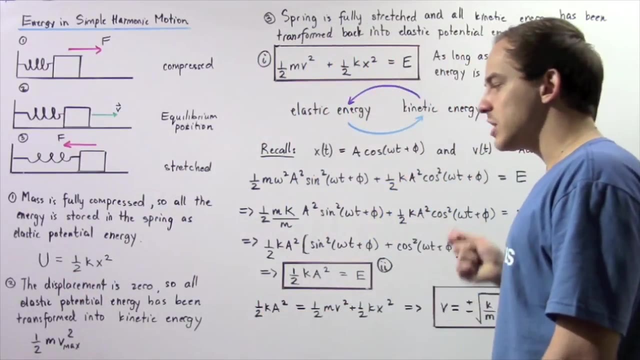 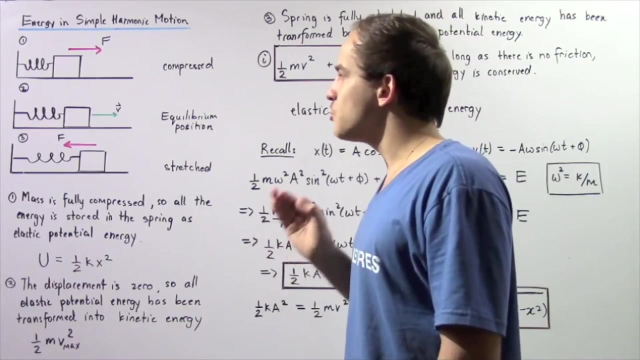 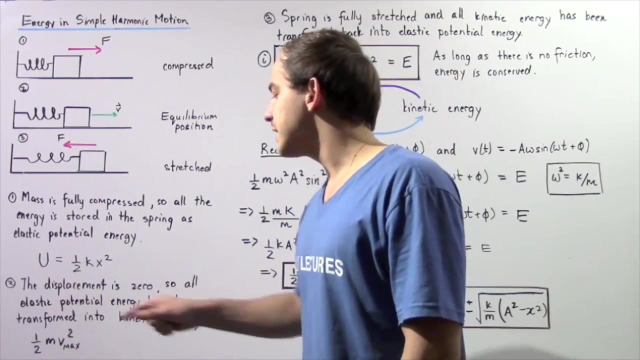 energy from diagram one, from our object being in this position, has been transformed into kinetic energy. that energy gave our object velocity. so at diagram two the displacement is zero. so all the elastic potential energy has been transformed into kinetic energy. and to calculate how much kinetic energy we have at the equilibrium position we have to use the following formula: 1- half mass times. 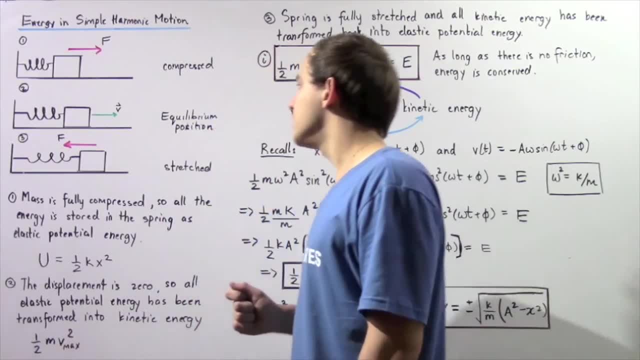 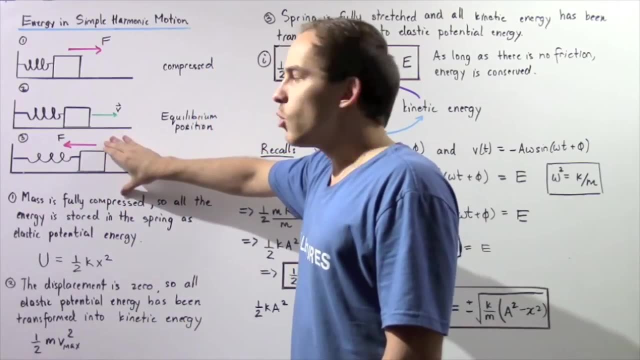 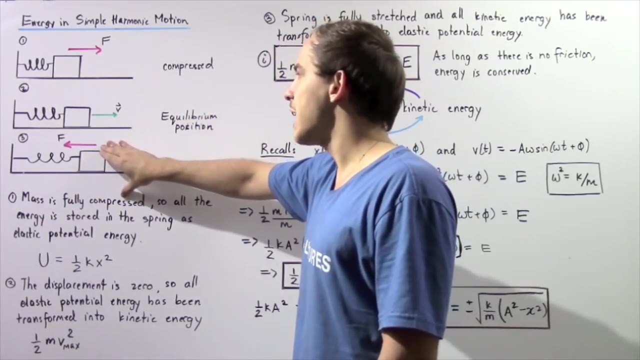 vmax squared, where v max is our maximum velocity. now, what about when our object is stretched? when our object reaches this position? well, once again all that kinetic energy has been transformed into our elastic potential energy, whereas in this case we had elastic converting to kinetic energy from, again, our potential energy from object, the stretched Turbo t in our object. 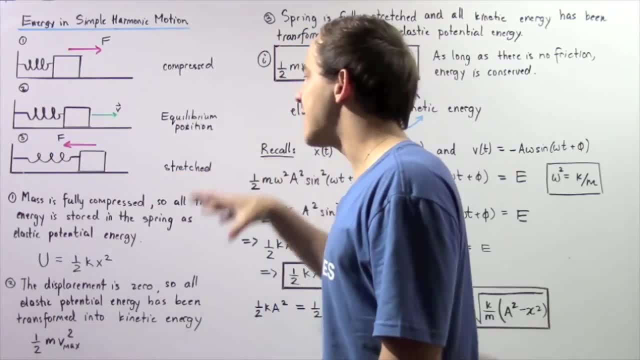 each time user Простоeta a energy is 무 balance and itsee mass x isrophatic energy protein n習 Lab of mass. stop all means. the action of the mas procures will be lost. so the mass in the strangers kinetic. in this case we have kinetic converting to elastic potential. 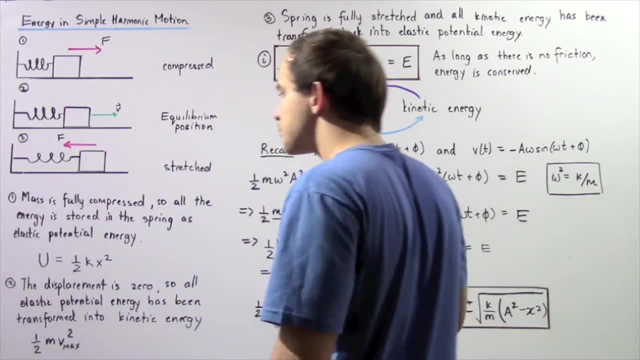 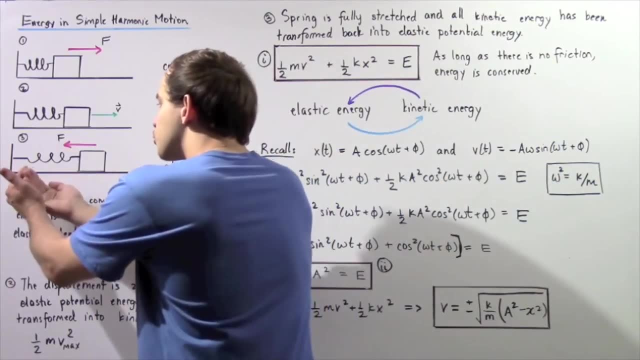 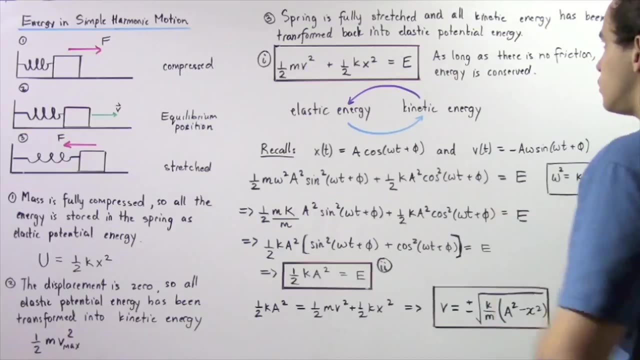 So let's suppose our object is stretched a certain distance. that means, if we want to calculate how much elastic potential energy is stored in this stretched spring, we simply use this equation. So once again, spring is fully stretched in position 3, and all kinetic energy has been. 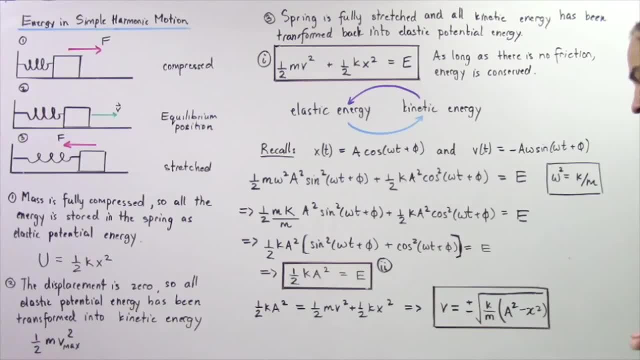 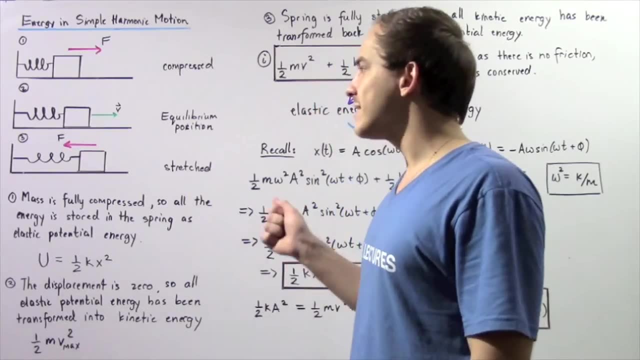 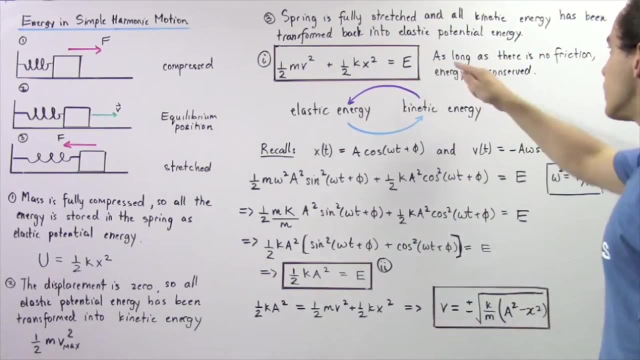 transformed back into elastic potential energy. Now, as long as we assume there is no force of friction acting on our mass and the spring, well then the total energy of our object is conserved. So, as long as there is no friction, energy is conserved and we have the following equation: 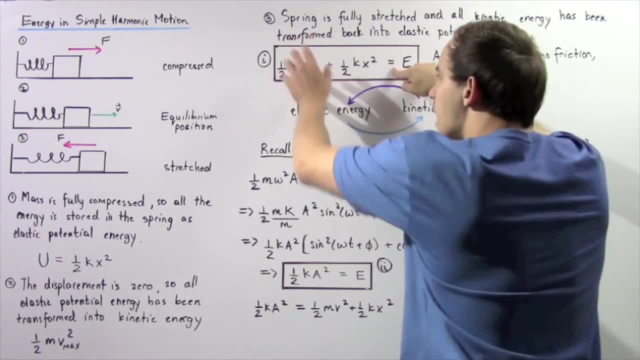 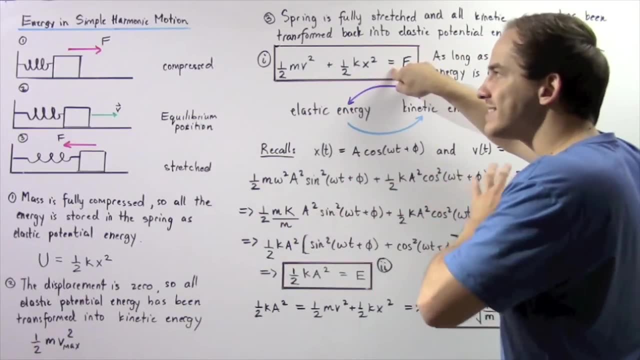 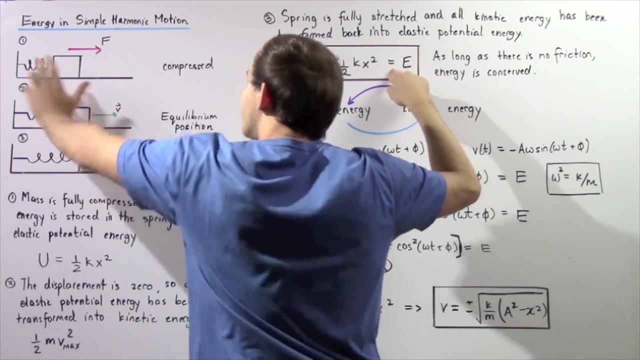 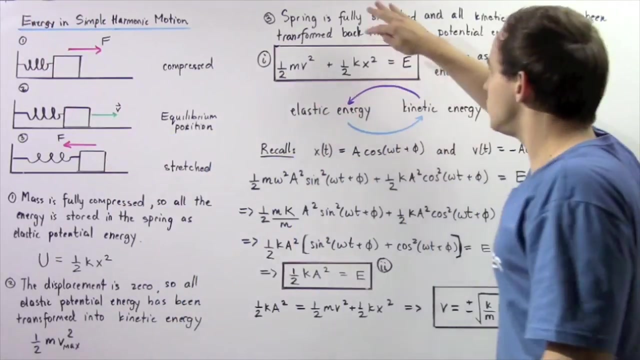 So the total energy is equal to the sum of the kinetic energy and the elastic potential energy of our object when the object is oscillating back and forth. So for example, at position 1, our object has no kinetic energy, So this term goes to 0, and the total energy at position 1 is simply 1 half k multiplied. 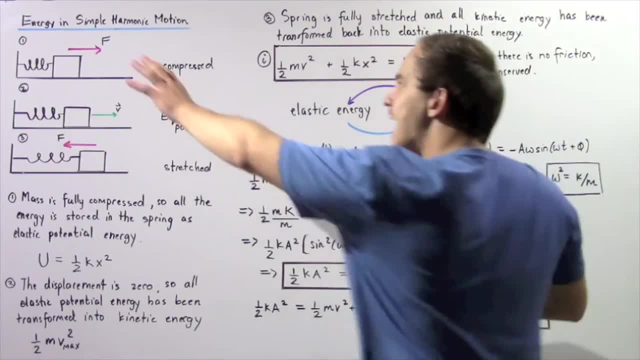 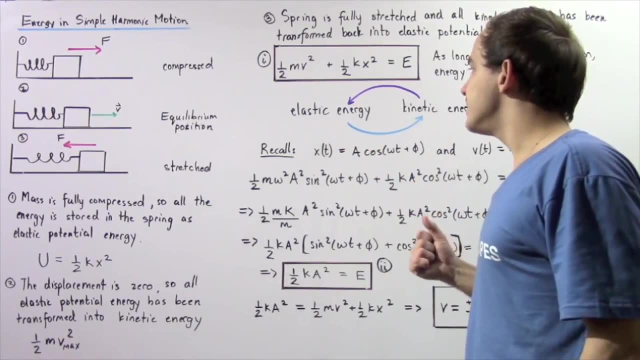 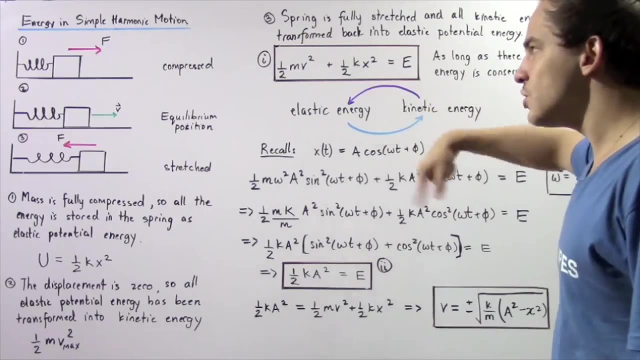 by x squared, where x is the amplitude of our harmonic oscillation. So our elastic potential, energy is 0.. Energy is transformed into kinetic, and then kinetic is transformed back to elastic, and the cycle continues on and on as our object is oscillating back and forth in simple harmonic 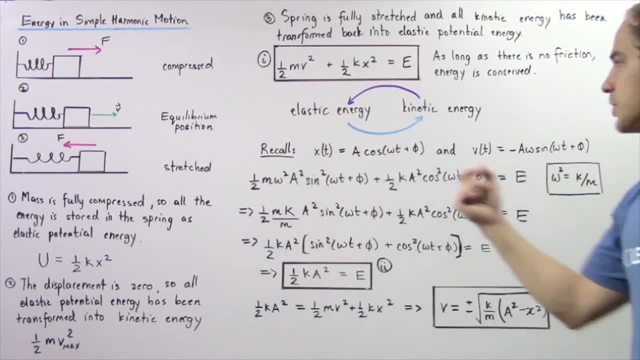 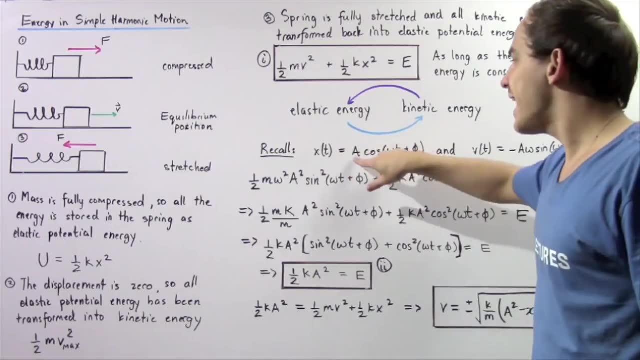 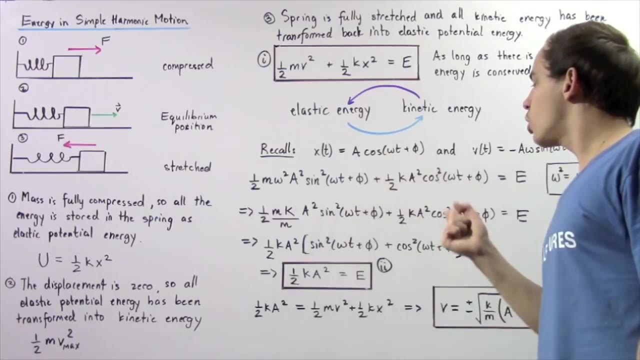 motion Now recall the following two equations. This equation gives us the position of our object with respect to time, So it's given by A our amplitude multiplied by cosine, of this quantity in terms of the velocity inside our cosine, So our angular frequency and our phase angle and our time t. 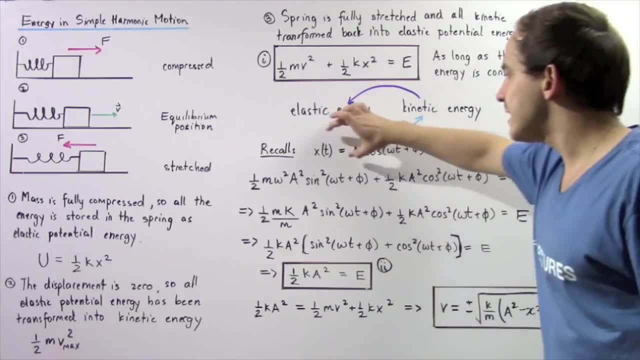 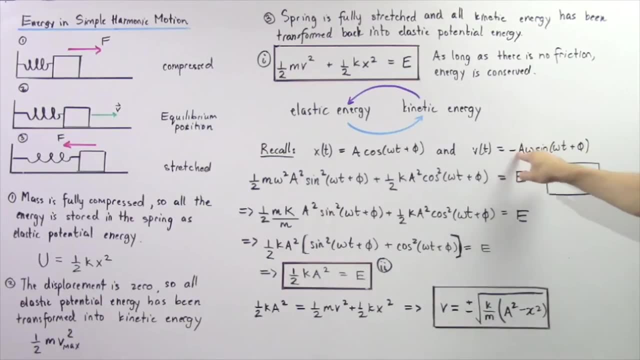 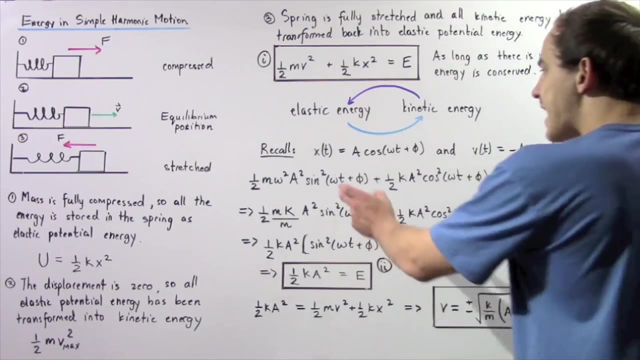 Now also recall that the velocity which is given by taking the derivative of this position function with respect to time, is given by this equation: Negative A, our amplitude, multiplied by omega, multiplied by sine of this quantity. So we can take this and plug it into the x in this formula and we can take this velocity. 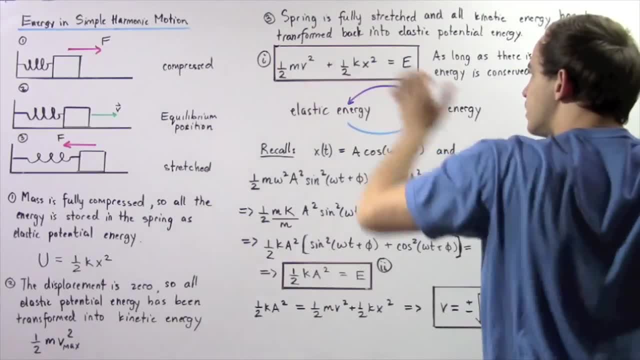 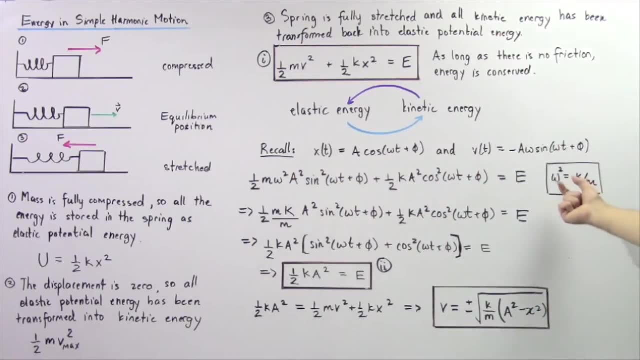 and plug it into the x in this formula, And we can plug it into the p in this formula, And plug it into the y in this formula, And plug it into the y in this formula And let's see what we get. Well, we get the following result: 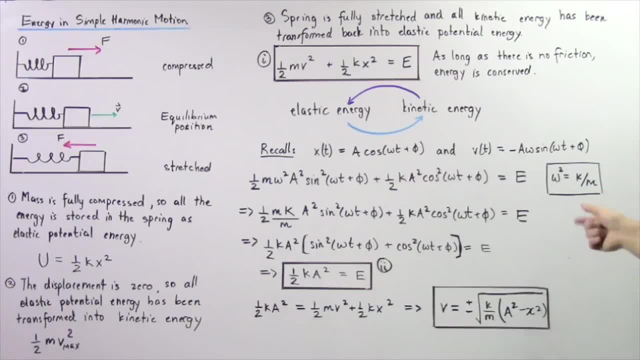 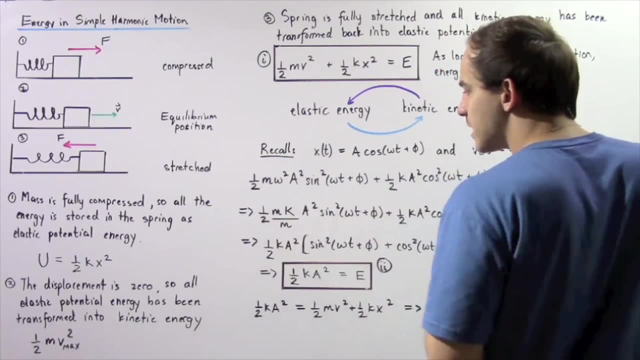 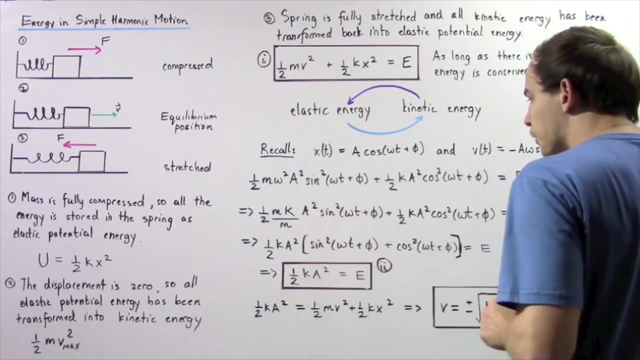 Now recall that our omega squared, the angular frequency squared, is equal to the ratio of the spring stiffness constant to the mass. So we can plug this quantity into the omega squared and we get the following result: have consistent terms appearing on both of these terms. So we have the k, the one-half and the a. 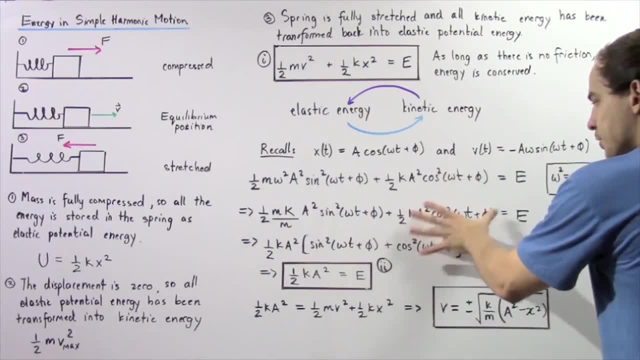 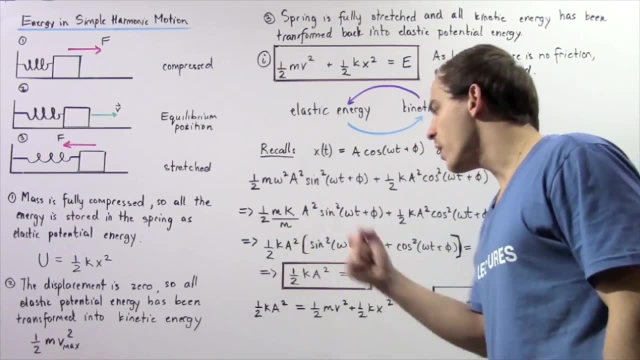 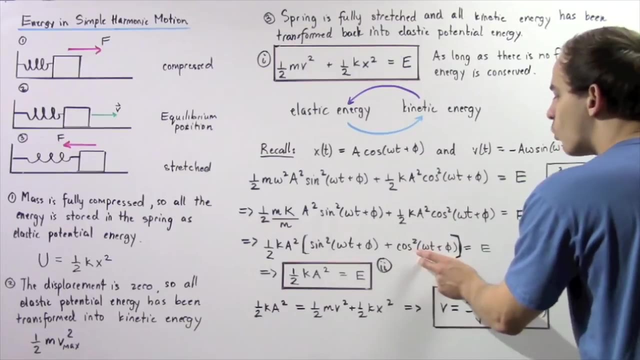 squared appearing on this term as well as on this term. So we can take those out and we get the following result: One-half k times amplitude squared is multiplied by sine squared of this quantity plus cosine squared of the same quantity. Now recall our trig function identity. It's